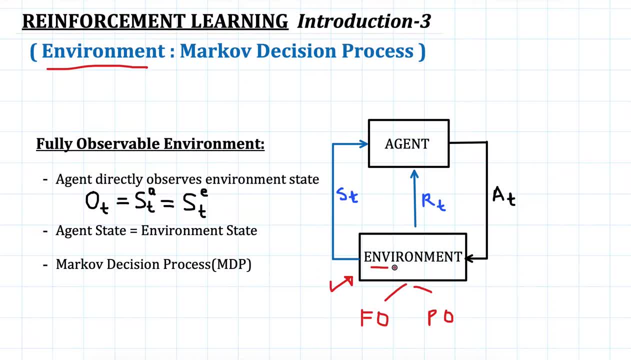 so. so there is nothing hidden inside the environment, so agent can completely see what's going on within the environment, and so it can directly use environment state as its own state. so here in this case. so observation at time T would be the same at state at time T. so because 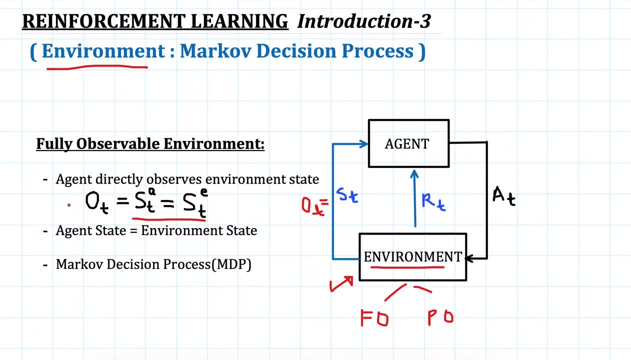 nothing is hidden from the agent and the agent does not need to construct its own representation of how environment is functioning. it's given that model, like if we are creating an agent which is trying to learn some game and we are feeding the exact rules of the game to the agent beforehand. so it's not the job of the agent to figure out what- uh, what's going? 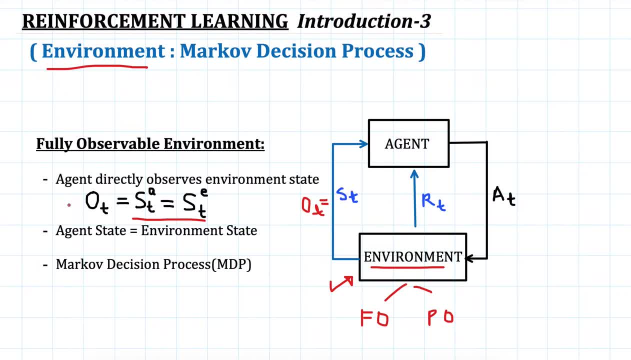 going on, but we have given out how the environment functions. everything is clear. so whatever is the observation in time, step T, that it can use as its own state, so agent state is same as environment state and this is the formally definition of Markov decision process. so this is the good case where agent state is same as 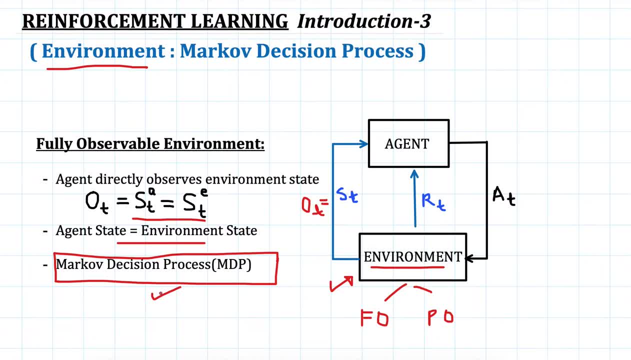 environment state or the world state, and this formalism is known as Markov decision process, and we will use this a lot throughout our reinforcement learning. now the other case. we will use this a lot throughout our reinforcement learning. now the other case. we will use this a lot throughout our reinforcement learning. now the other case. 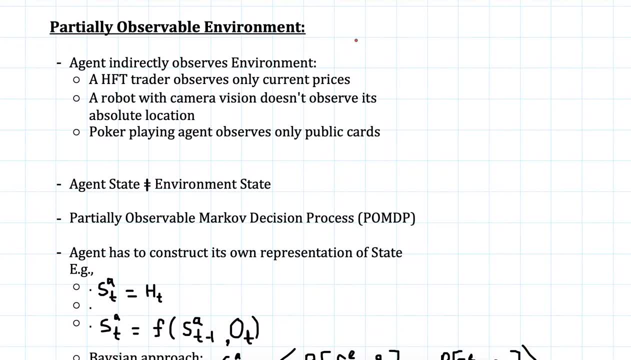 indirectly observes the environment, partially. it only partially observes the environment. it does not have a clear picture of what's going on in the environment. so one example could be a high frequency trader. so the trader, uh, who is trading at very high frequency, it's not an investor, he is a trader. 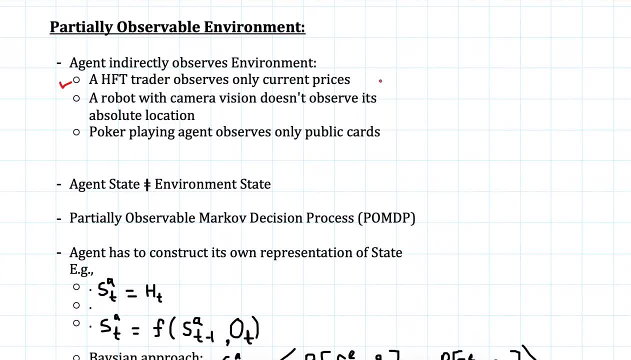 and uh, the algorithm that is being used there looks at only the current prices, so it's not concerned with the historic prices of the stock market. it looks a very small region which is close to the current price and it only observes that price. it it has no uh data about what's what was. 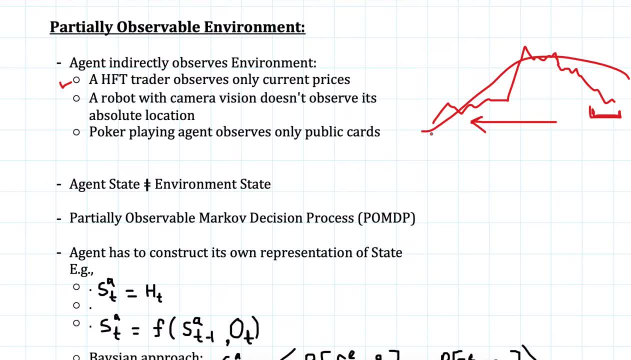 the trend. what is the trend? and uh, how has the stock? uh behaved in different situations? so this trader trading algorithm has a very narrow view. it observes only a small, small part of the environment, not the complete environment, similarly a robot who is learning to walk, so so environment may be a very complex path. 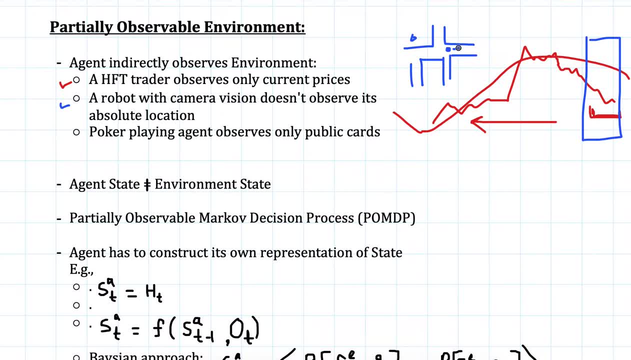 but the robot is walking current currently here, so it it has a camera vision and it observes very limited part of the environment and it it will make decision based on that. it will not know that, uh, if it goes 100 meter ahead and then go left, then there will be again. 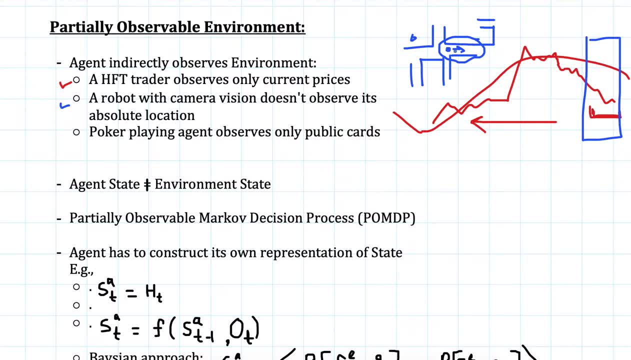 a left turn. it has no idea about that. it has to, uh, take decision based on whatever it can observe, so it has a very partial observation about the environment. similarly, a poker playing agent observes only the public cards that is shown and not the card which are to the 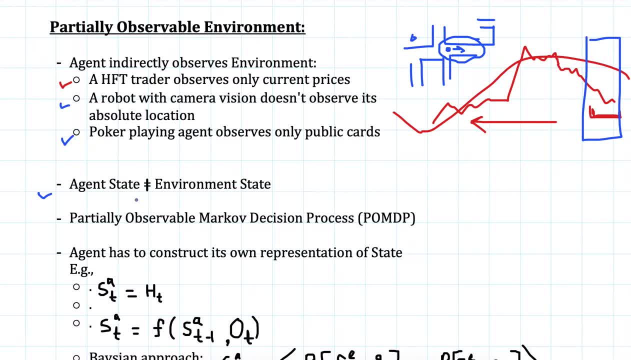 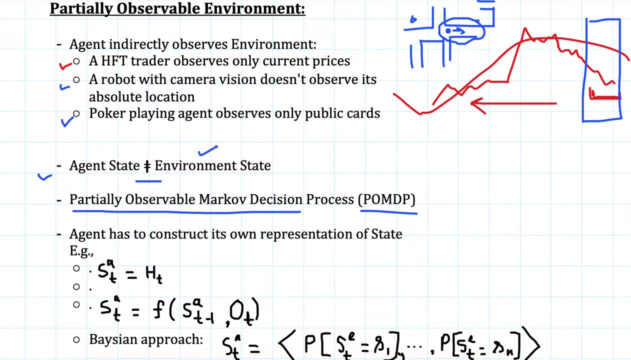 players. so in this case agent state is not the same as environment state and formally this is the definition of partially observable Markov decision process, or in short, POMDB. so since agent cannot use the environment state because it does not have a clear vision of what's going on inside the environment, it has to construct its own representation. 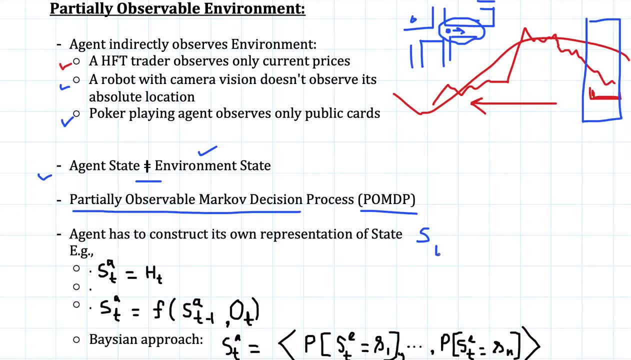 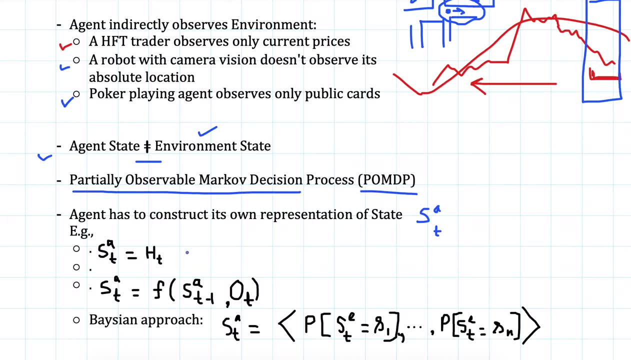 of the state, of the agent state, so it can construct its representation of the state in various ways, like one way could be to take the entire history as its state. so whatever value it has observed or whatever rewards it has got till time, step t, it will consider. 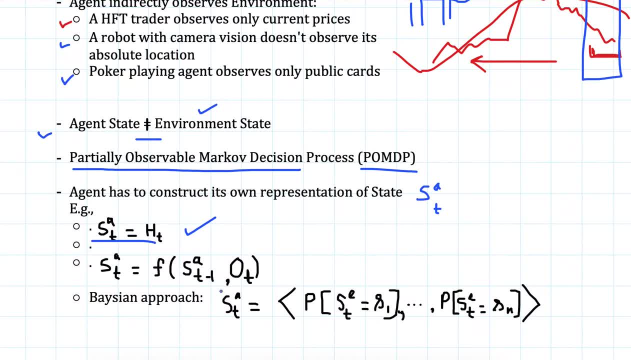 that as a state, that is a valid representation of state and other can be that it takes a probabilistic approach or Bayesian approach, where it assumes what's the state of environment at time t. so with probability this p1, the state of environment is s1 and similarly with probability pn. so 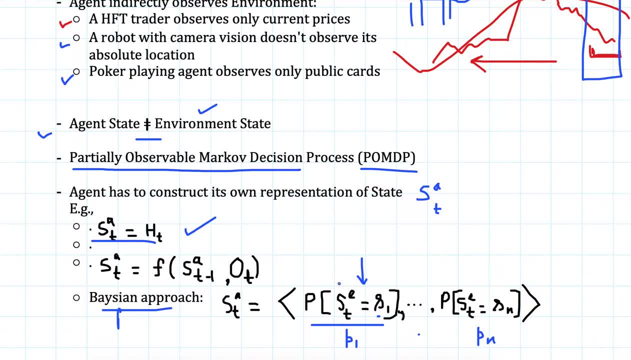 it does not construct exact representation of state, but it takes a Bayesian approach. then what is the probability that environment state is s1, p1? so this is sum of all p1 to pn should be one. so it creates a Bayesian or probabilistic approach and it constructs view of environment. it guesses. 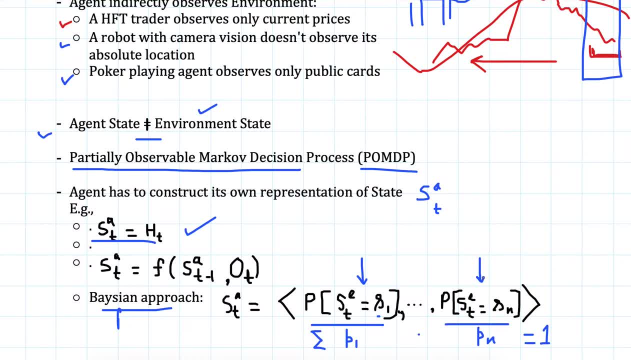 what the environment is. environment state currently is. each and another way could be. it defines some function which depends on its previous state, so it defines some state in the previous time step. but it received some observation OT which changes its assumption about whatever state it has defined, so it will modify. 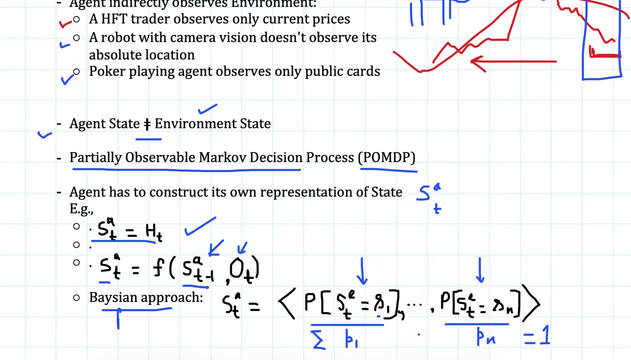 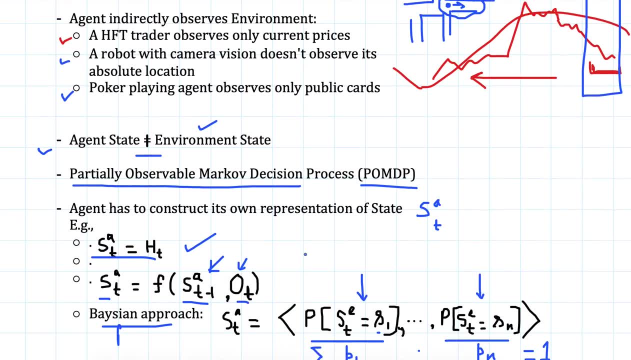 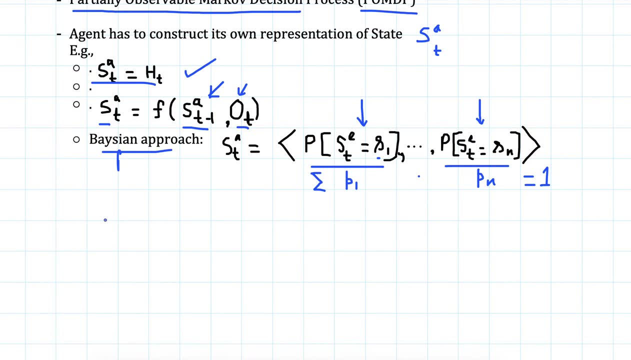 its current state, depending on what was the previous state and the new observation. and another example to make it more clear would be, like many people play games on the mobile phones, like if we have a game. today we have a game which is very popular called temple run. 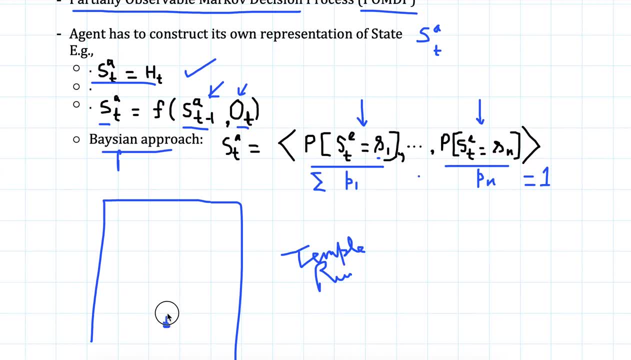 so here the agent is running and it's faces several obstacle like sometimes it may face some fire. in that case it has to jump over that and in other case it may jump into water and then it may get a rock or something else or a piece of wood in its path. in this, 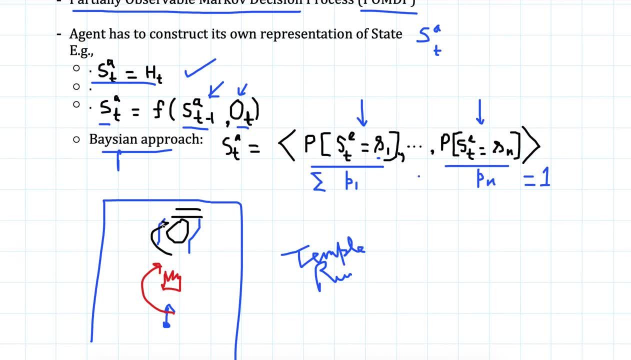 case, in case of a rock, it would have to jump or take sideways. in the case of this, on the top of this water, it has to just slide underneath that. so the agent takes its decision based on what it observes. it has only a very small vision of the environment and it does not fully observe what's going. 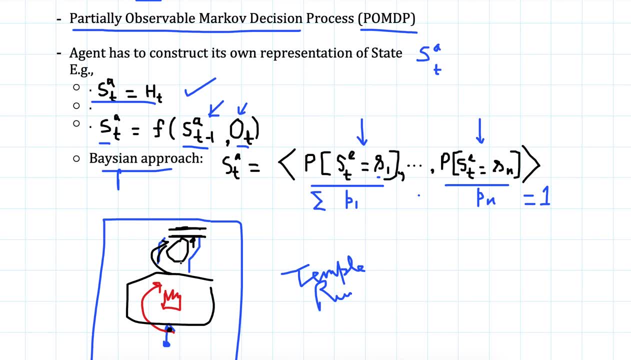 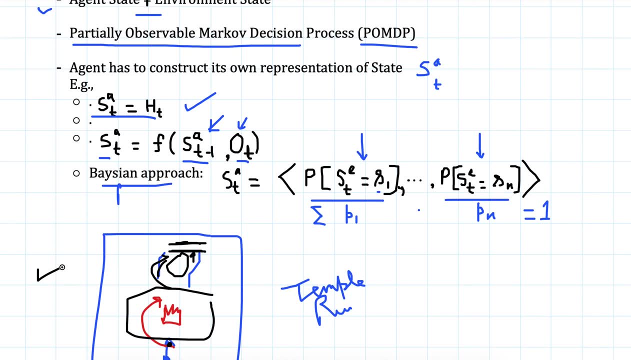 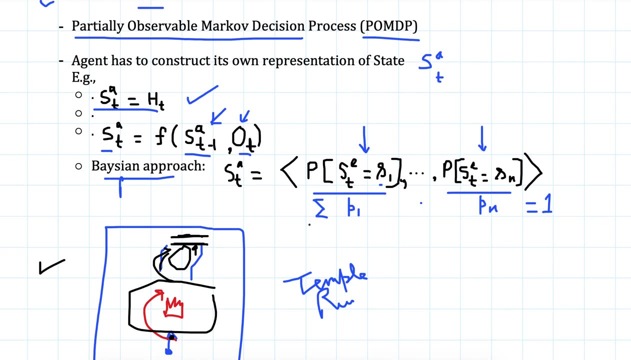 on. so how environment is deciding what next hurdle to add to the scene. so this is completely hidden from the agent. so this will also be an example of a POM DP that is partially observable Markov decision process. so that's it. I will end today's video with that and in next lecture we will focus on this agent parts.